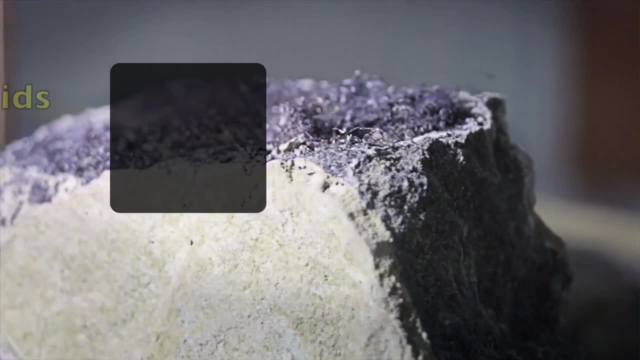 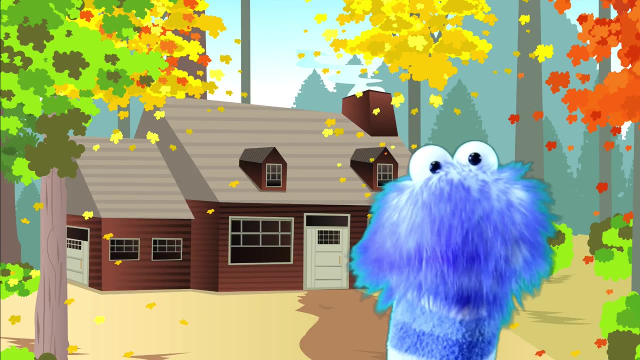 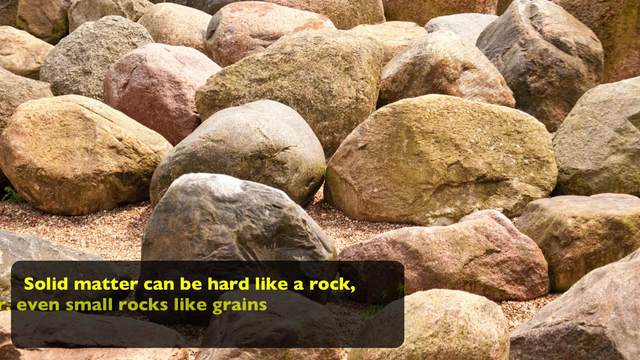 And there are different states of matter, and those states are solids, liquids and gasses, And plasma is another, but not as common, and we'll talk about that a little bit later. And solid matter can be hard like a rock, soft like fur, even small rocks like grains of sand and dust. 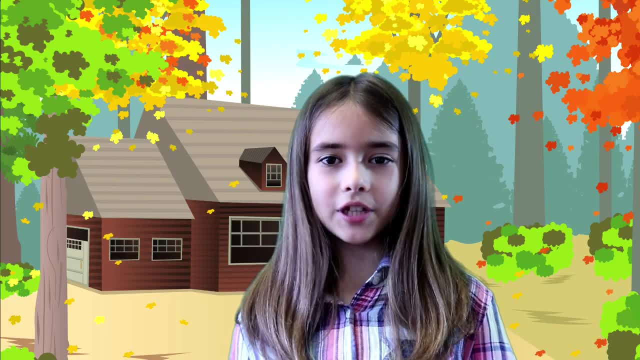 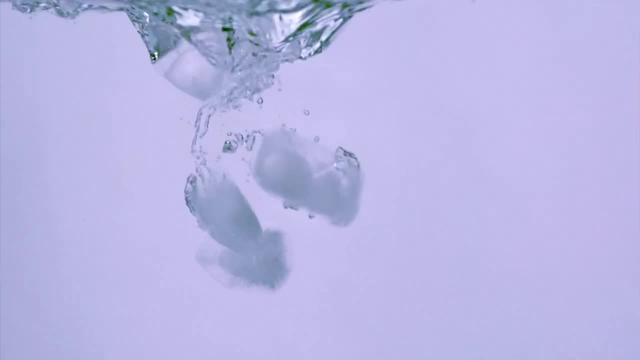 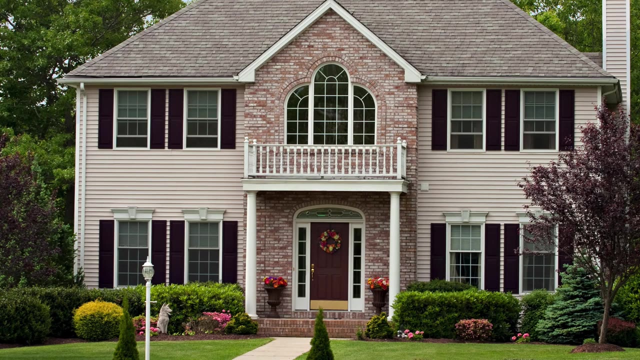 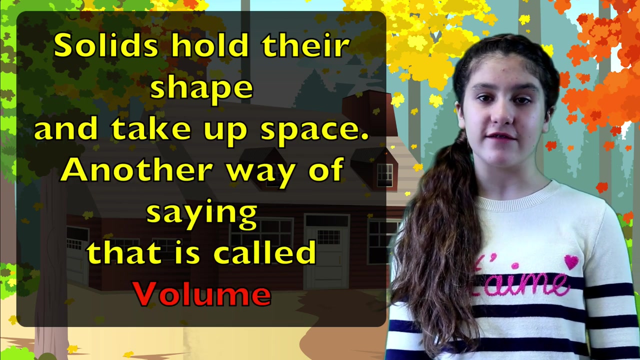 Solids are objects that keep their own shape. For example, an ice cube is a solid, but when it melts it becomes a liquid. And other examples of solids are trucks, books and houses. Solids hold their shape and take up space. another way of saying that is called volume. 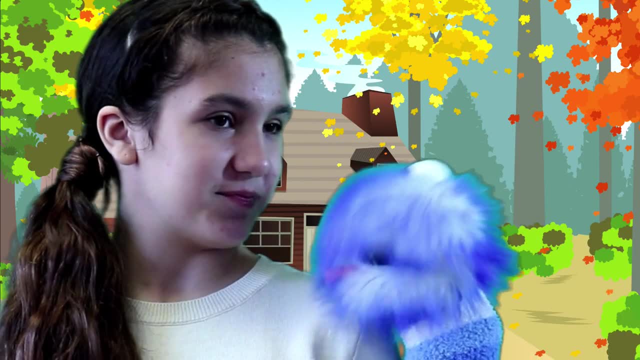 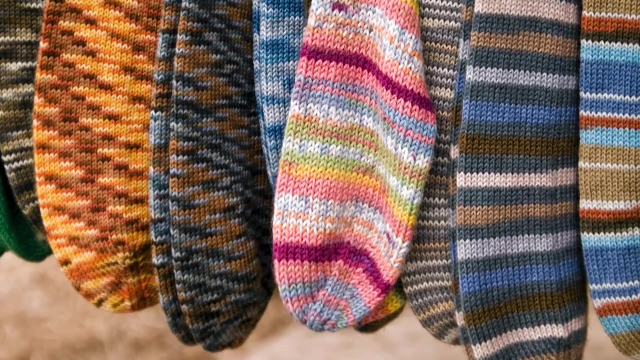 I must take up volume in the sock drawer because that's where they put me when we're not making videos. Sorry, Gus, that's just the best place to hide you. To be honest with you, I don't know how much we could deal with your voice all the time. 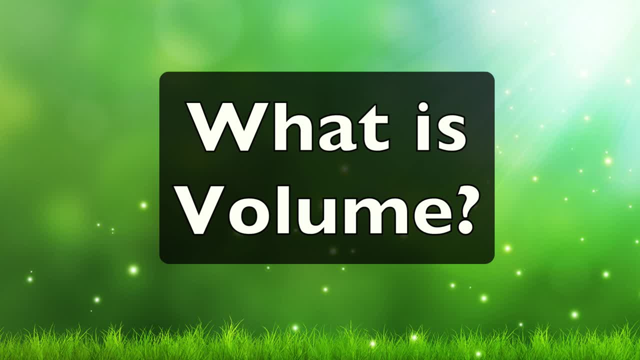 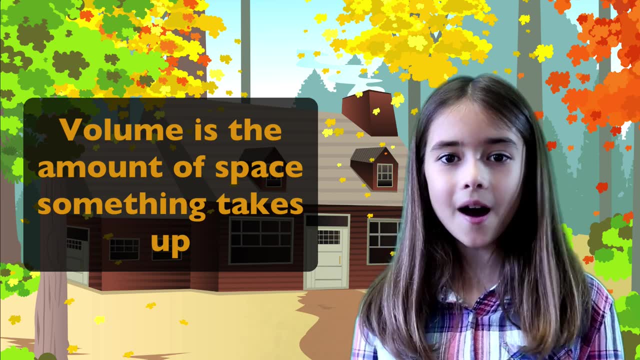 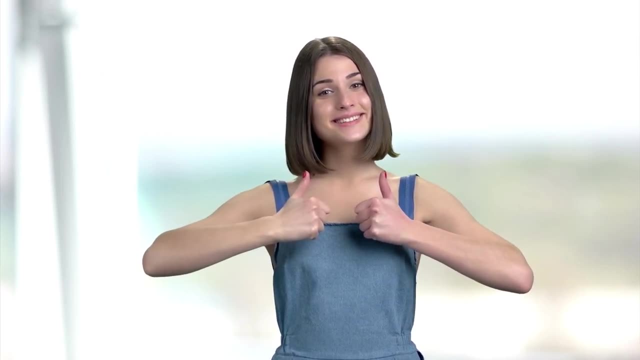 So the next question is: what is volume? Volume is the amount of space something takes up. And speaking of up, why don't you give our video a thumbs up if you like this video so far? It really helps get these videos out there to people just like you. 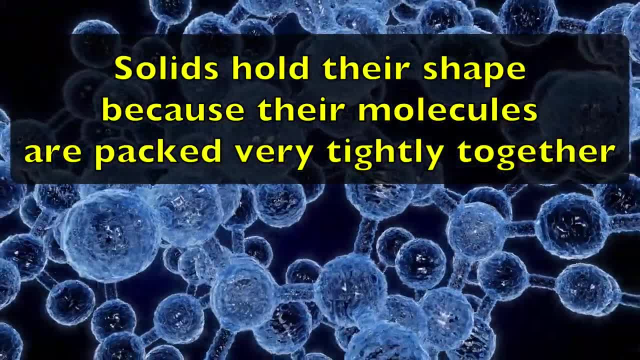 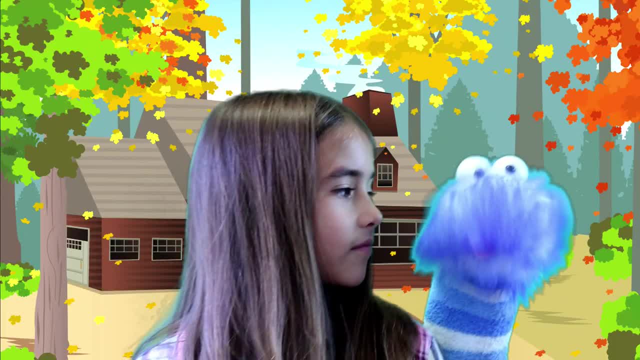 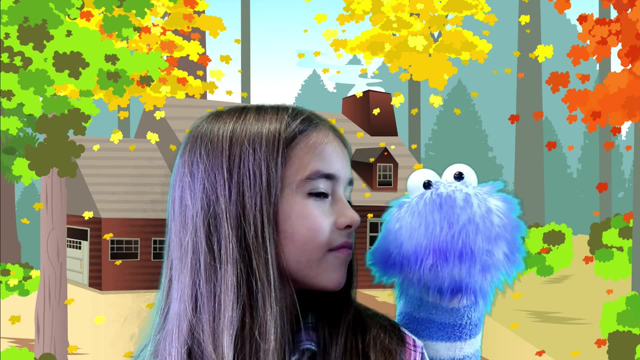 Solids hold their shape because their molecules are packed tightly together. Large solids hold its shape. the same way. The atoms inside of the solids are not able to move around too much because they're packed in tightly too. Wait, what are atoms? Let's find out. 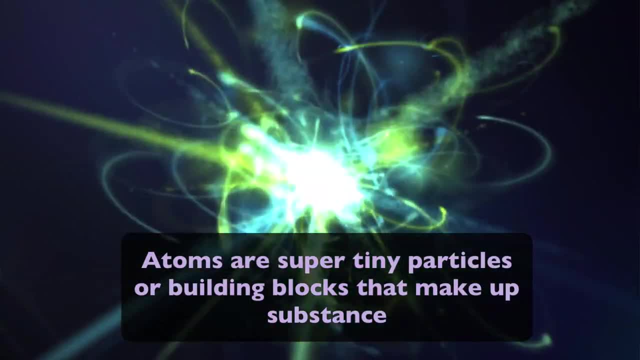 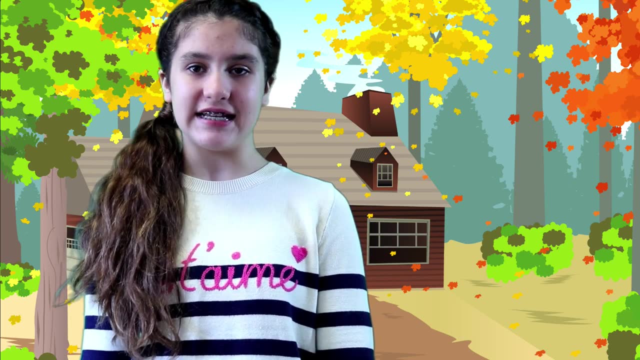 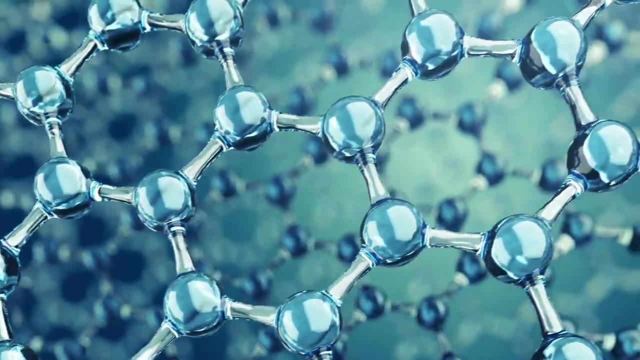 Atoms are actually super tiny particles or building blocks. Atoms are actually super tiny particles or building blocks that make up a substance. The atoms in liquids or gases bounce and float around easily wherever they want, But the molecules in a solid are stuck. 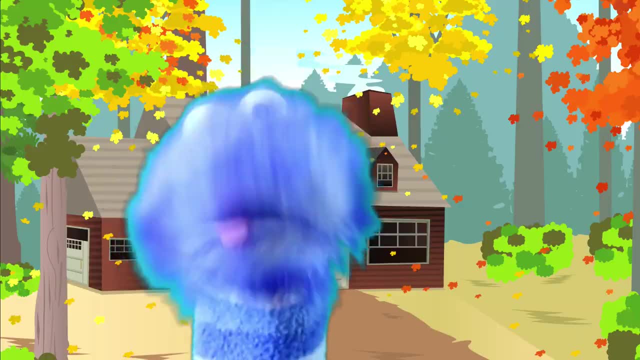 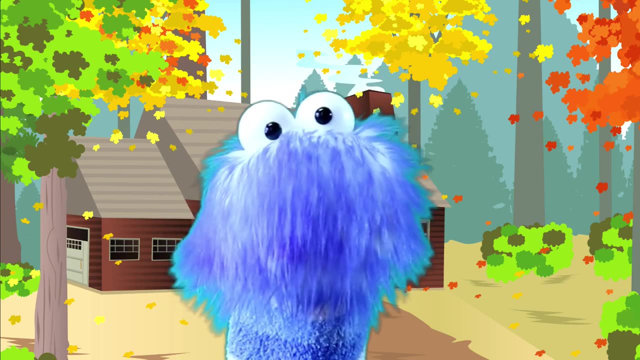 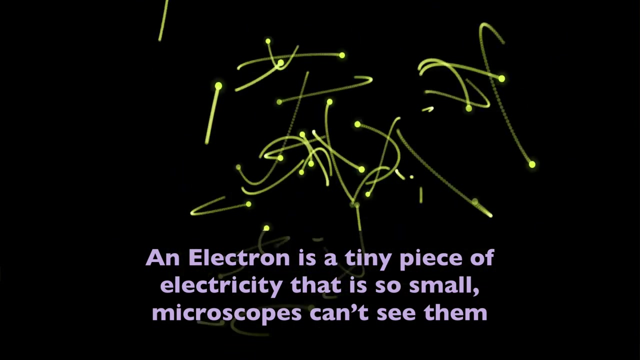 and can't really move. And the atoms still vibrate and electrons move around, but the entire atom will not move at all. An electron is a tiny piece of electricity that is so small microscopes can't even see them. Next we have liquids. 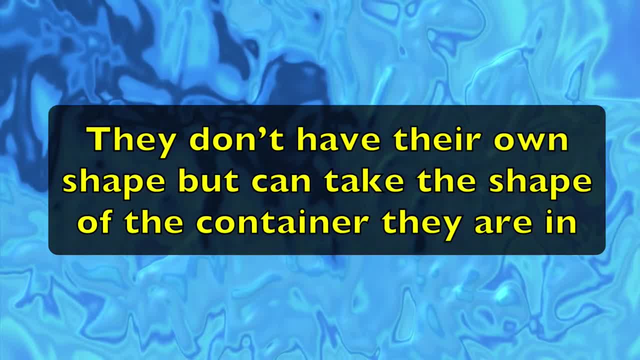 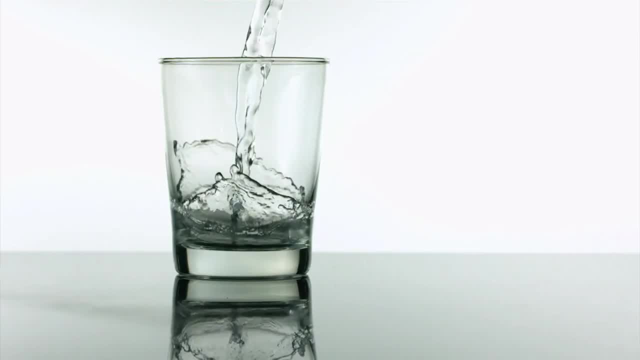 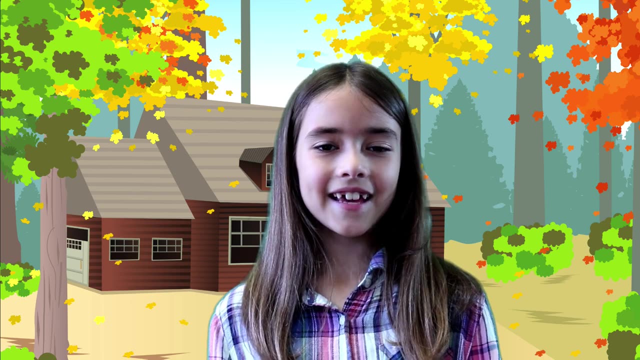 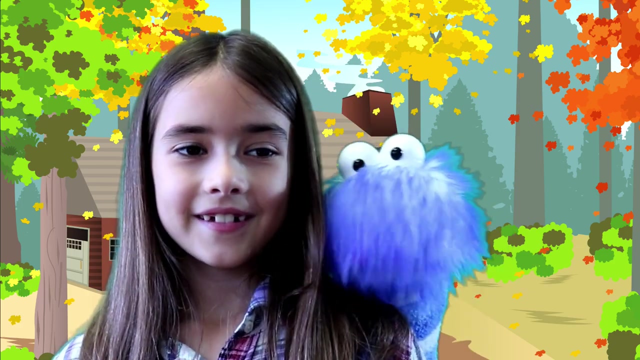 And liquids don't have their own shape, but they can take the shape of any container they're in And they can also flow at a different temperature. Examples of Examples of liquids are juice, water and coffee- Coffee- I like coffee. 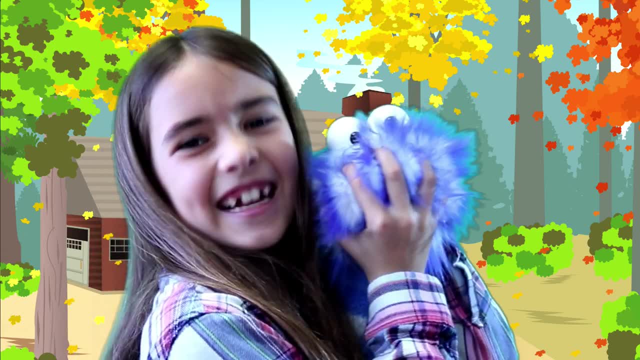 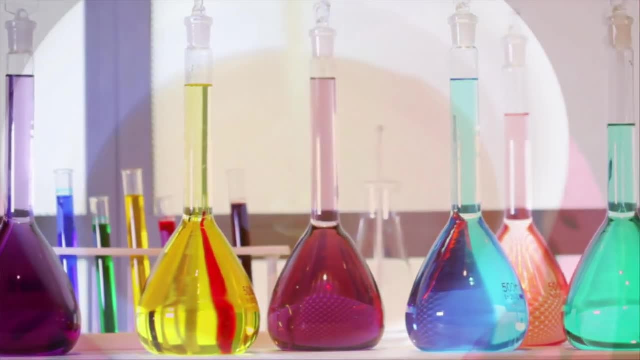 When they do let me out of the drawer, I'm like, I'm like. I'm like He has coffee Not a bit. And liquids can be different colors and thickness. For example, honey is thicker than coffee and also moves a lot slower. 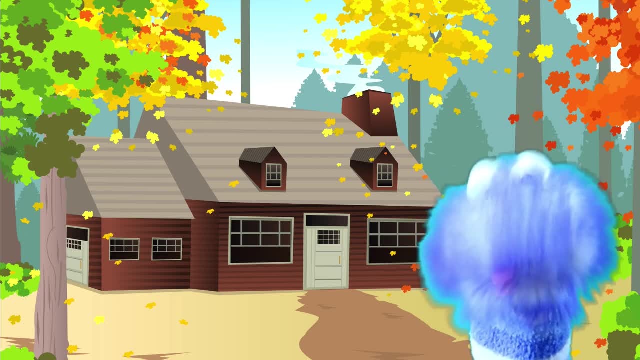 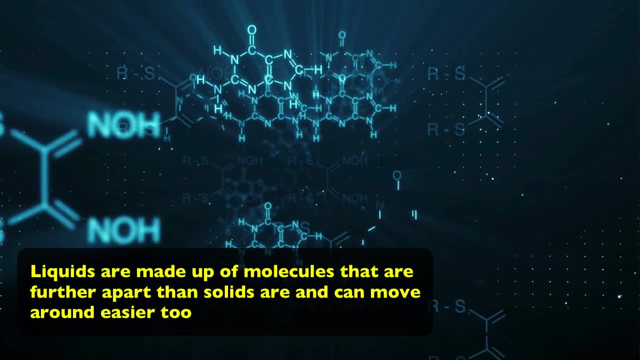 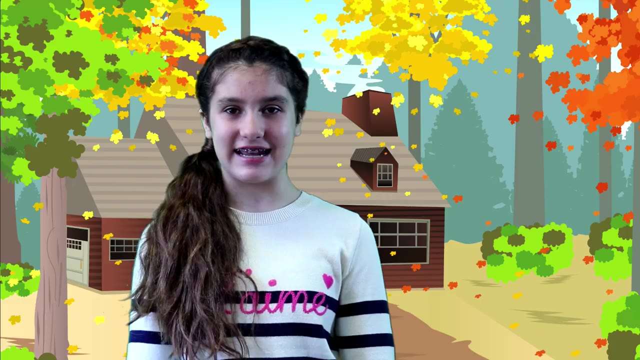 And you can measure liquids in a cup or a spoon, And liquids are made up of molecules that are further apart than solids and can move around a lot easier too. Liquids are found in the middle of the solid and gas states. Gases are air-like substances. 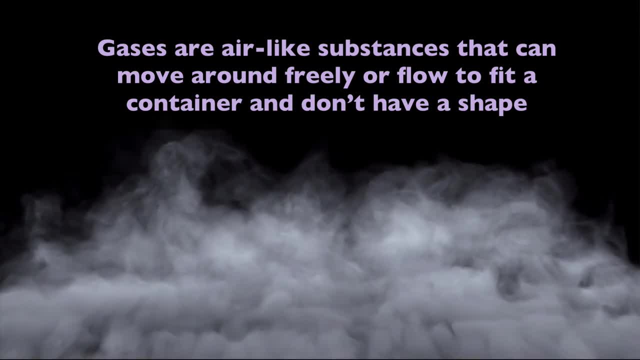 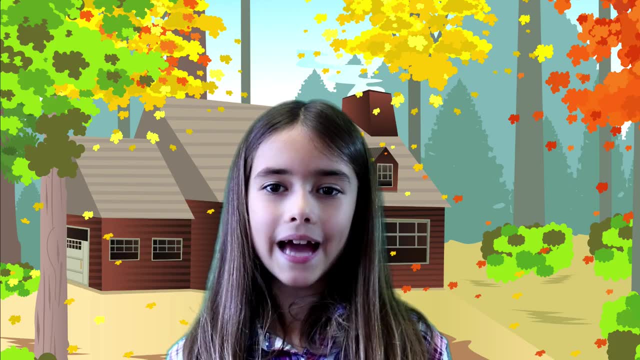 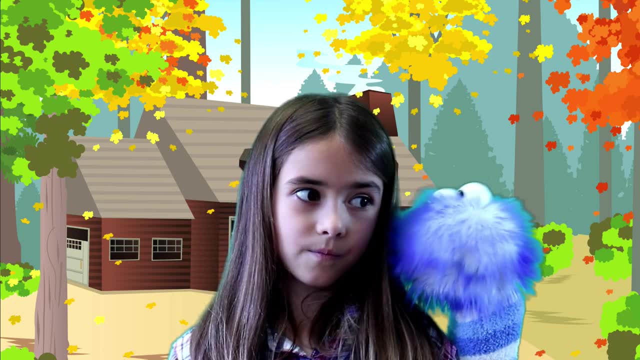 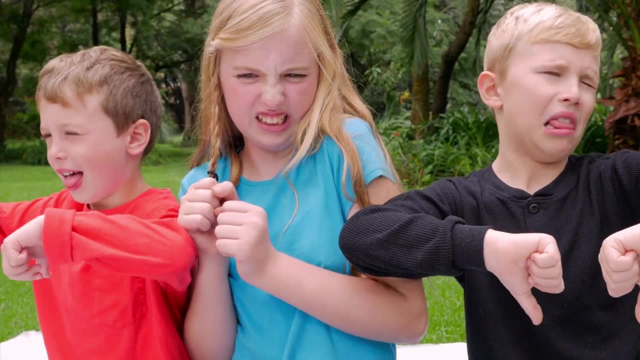 You can walk through gases and won't feel them. I've walked through gases before, right behind you, and I've smelt them. Maybe cadence instead. just That's a different type of gas, Gus, That's a natural gas. That's my dad joke. 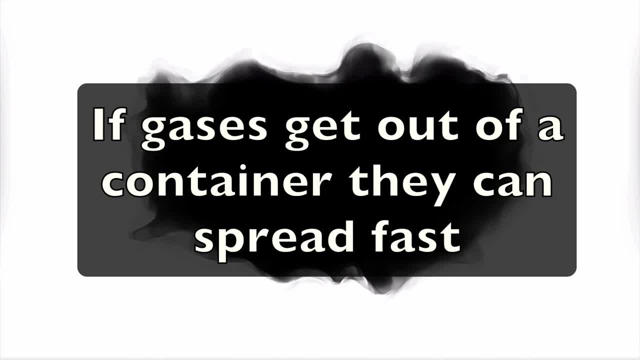 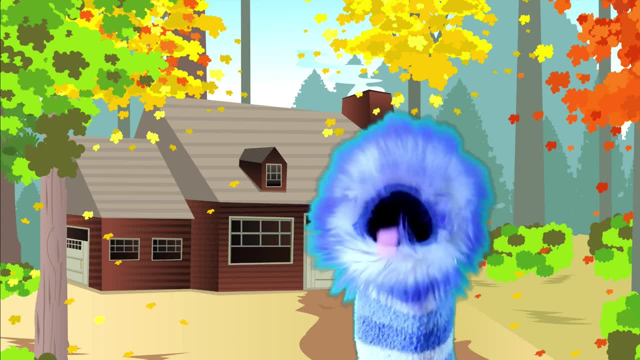 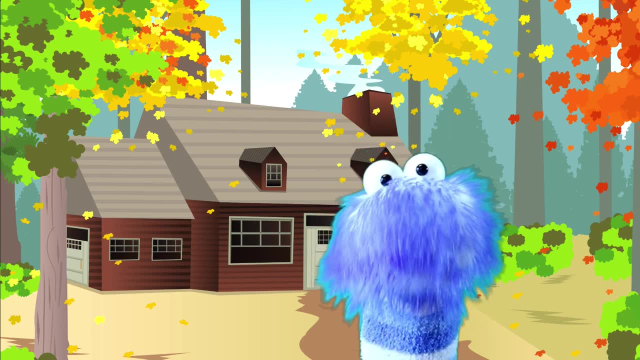 Anyway, if gases get out of a container, they can spread fast. Gases are everywhere and surround us with the air we breathe. They float around you or can be trapped in bubbles. In fact, the studio where we film these always smells like gas after the girls leave. 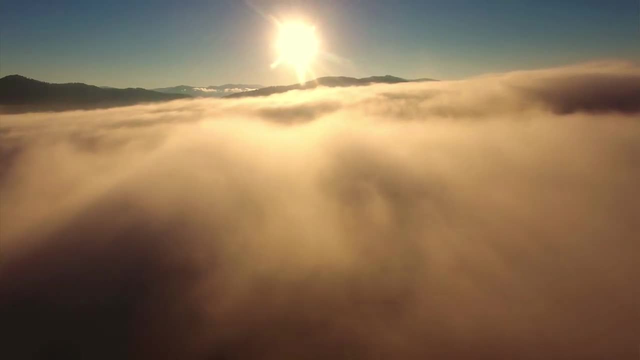 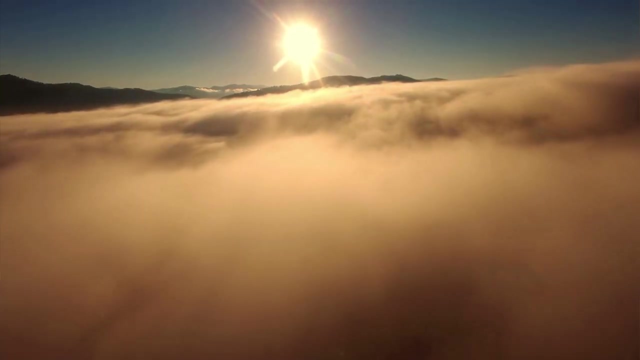 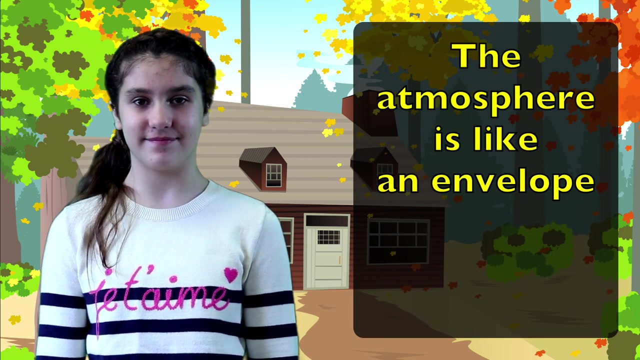 Oh, Gus, you're gonna be in trouble with those girls. Well, let's move on. You may have heard of the word atmosphere. The atmosphere is like an envelope of gases that surrounds our planet, And molecules in gases are called molecules. 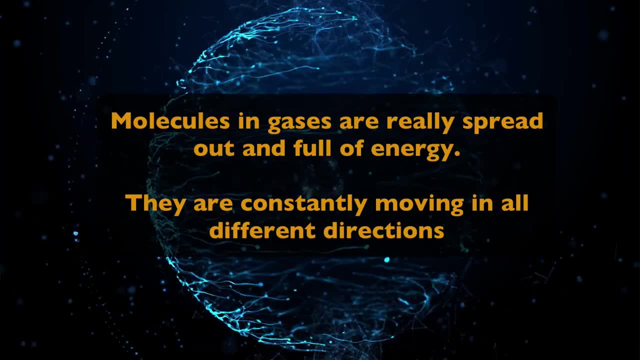 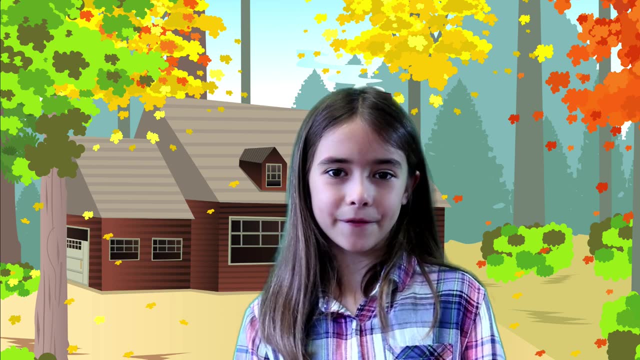 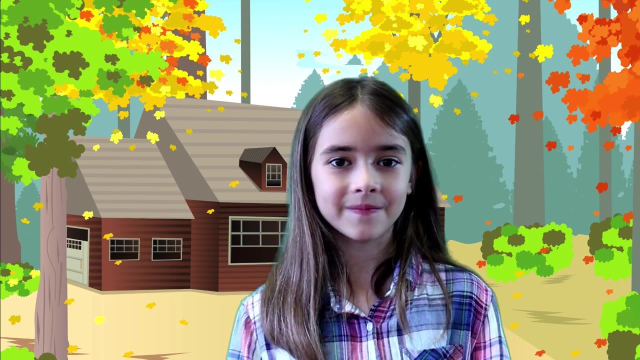 Gases are really spread out and full of energy. They are constantly moving in all different directions. Gases can fill any size container. It doesn't matter how big or small it is. An example would be like this: Think about a balloon. 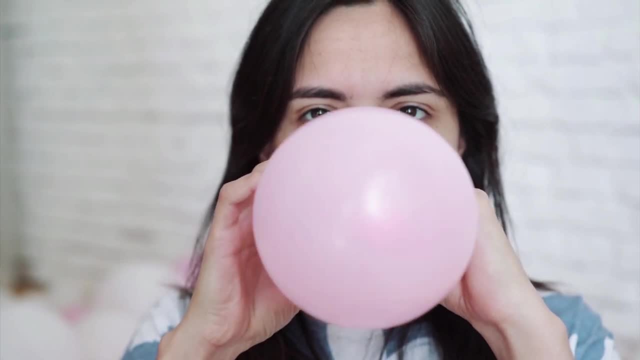 No matter how big of a balloon, even balloon animals, they will be filled with the gas molecules that are in it. They will be filled with the gas molecules that are in it. They will be filled with the gas molecules that are in it. 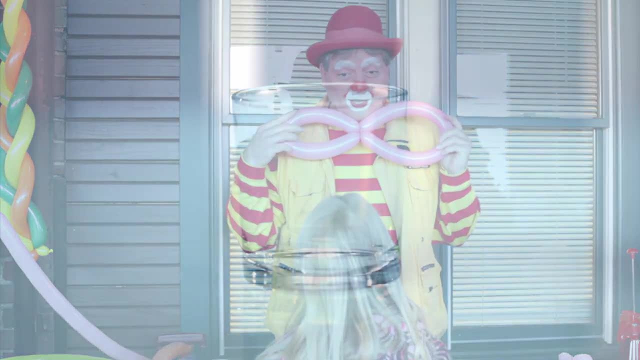 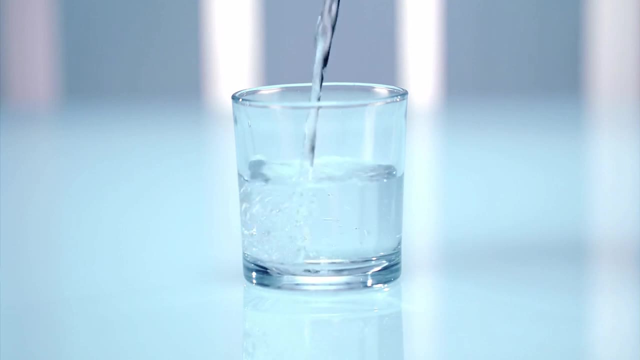 Evenly, all throughout it. Evenly, all throughout it. Liquids can only fill the bottom of a container, like a bucket, for example, And while gases will be able to fill it entirely. So now let's move on to the fourth state of matter. 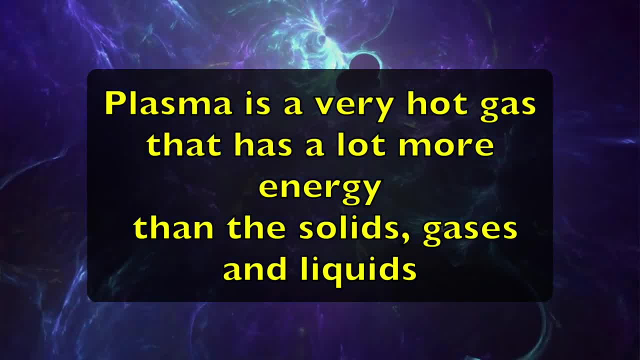 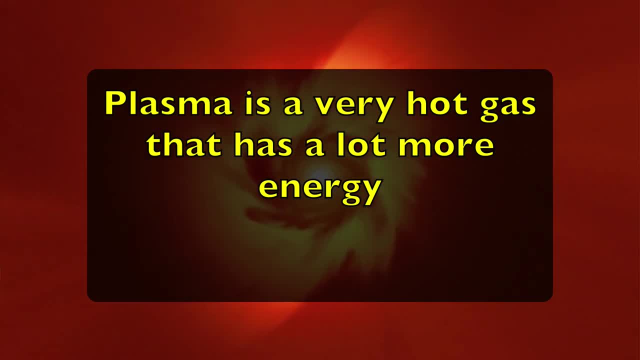 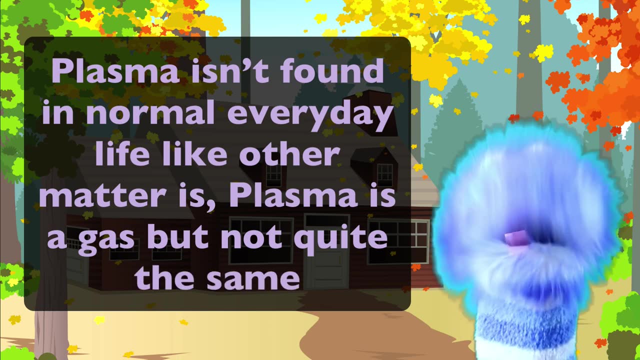 And plasma is the fourth state of matter. Plasma is a very hot gas that has a lot more energy than the solids, gases and liquids that are matter too, And plasma isn't found in normal everyday life like other matter is. Plasma is a gas, but not quite the same. 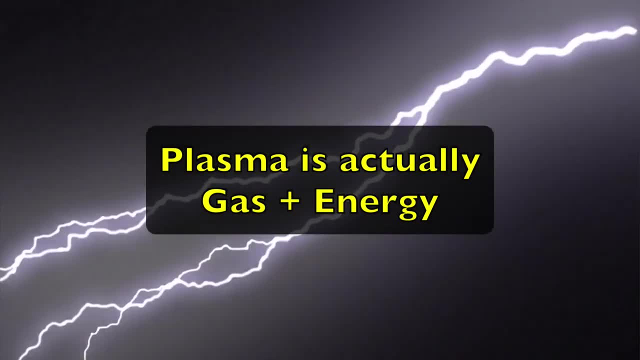 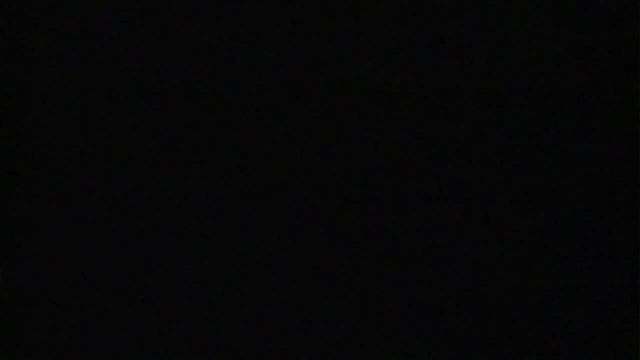 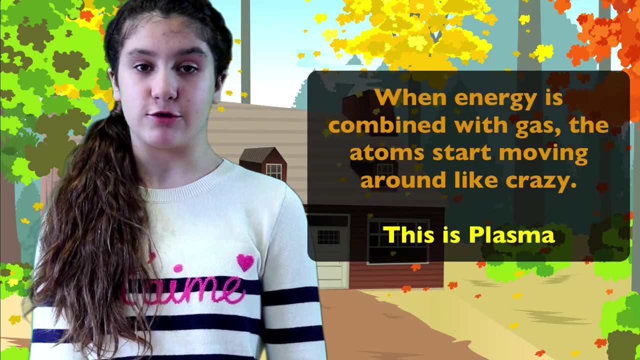 Believe it or not, plasma is actually gas plus energy. Think you've ever seen plasma before You actually have. If you've ever seen lightning in the sky, you've seen plasma. You see, when energy is combined with gas, the atoms in the gas, the atoms in the gas. 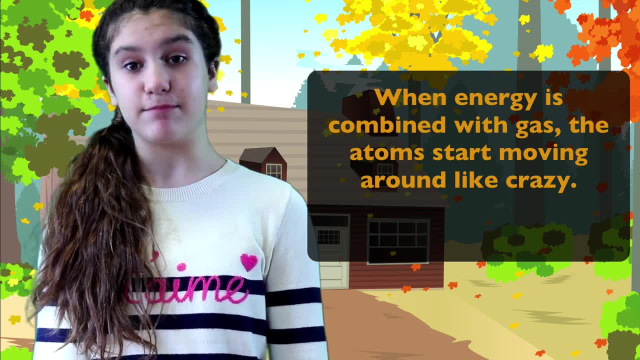 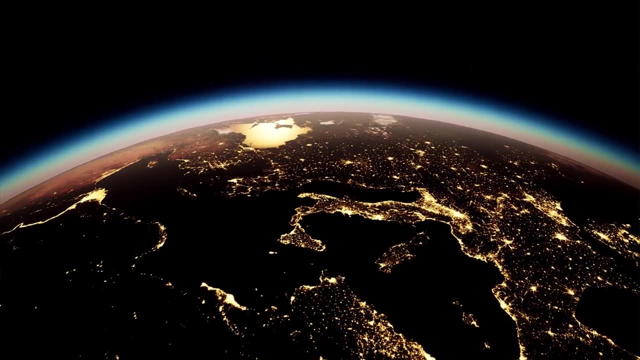 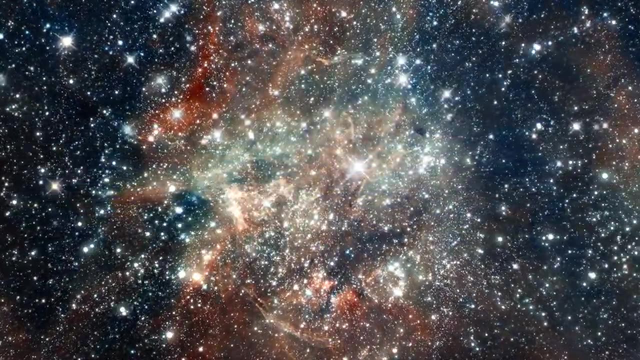 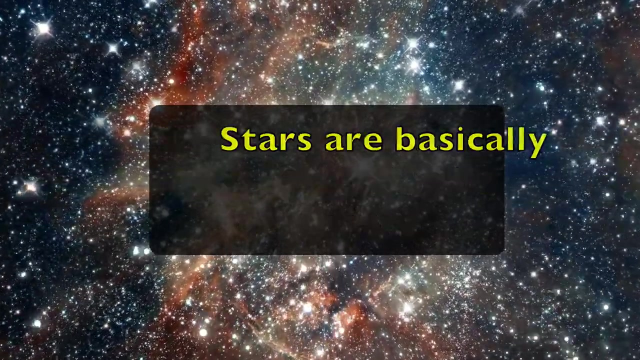 the atoms start moving around like crazy. This is plasma, And plasma is not a common state of matter here on Earth. However, plasma may be the most common state of matter in the entire universe Because, guess what? Stars are basically super heated balls of plasma.